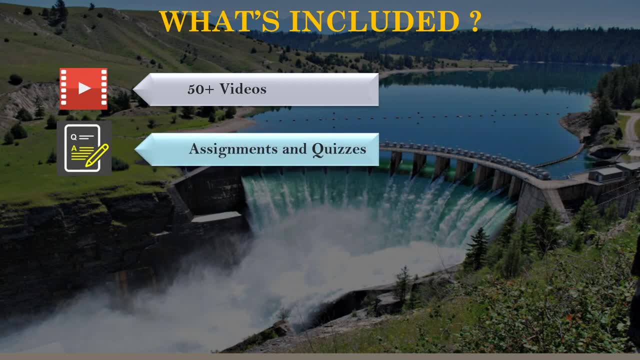 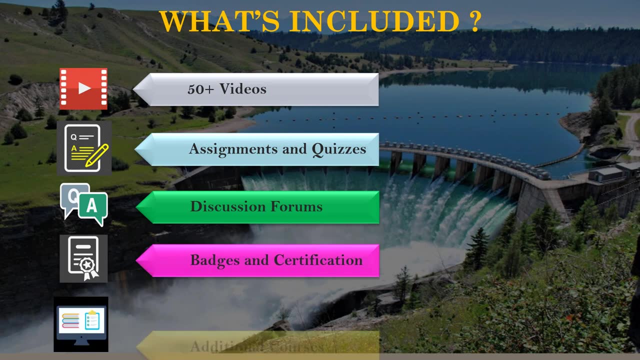 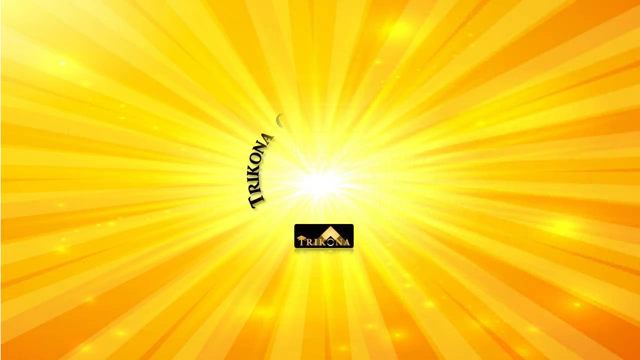 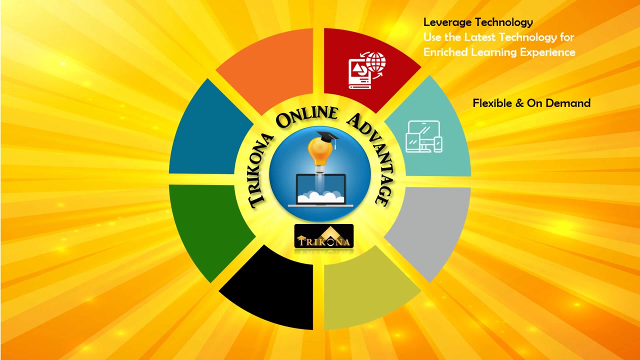 50-plus videos, Assignments and quizzes, Discussion forums, Badges and certification. Additional courses. Tricana Online Advice. Tricana Online courses come with many benefits, and these include Leverage technology, Flexible and on demand Self-paced Interactive. 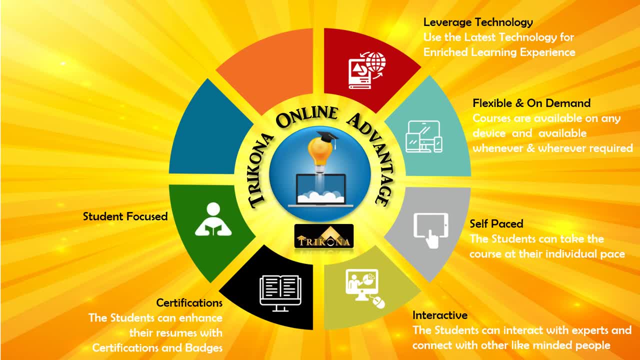 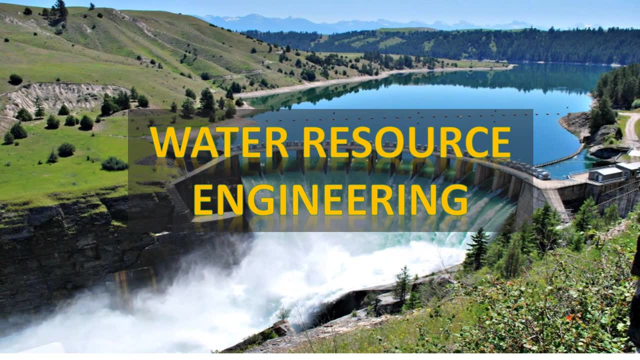 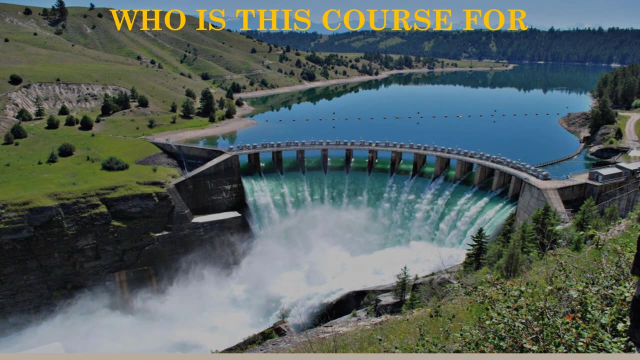 Certifications, Student-focused, Enhanced opportunities, Saved time, cost and effort. Water Resource Engineering. Who is this course for? This course is crafted for students who intend to learn the detailed aspects of water resource engineering. This course can be taken by BE or BTech Civil Graduate. 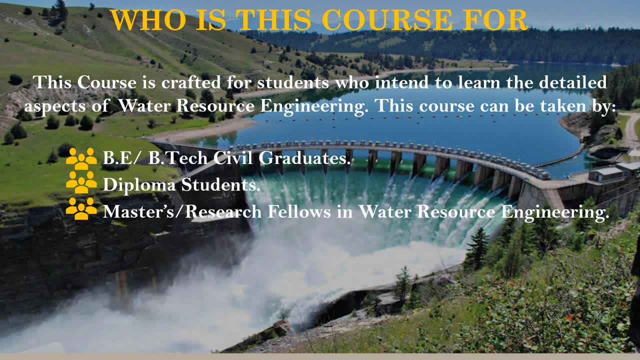 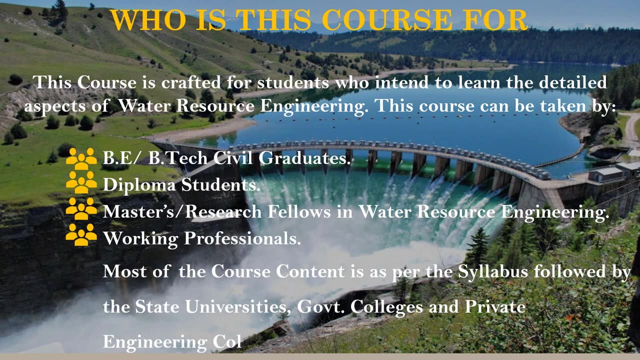 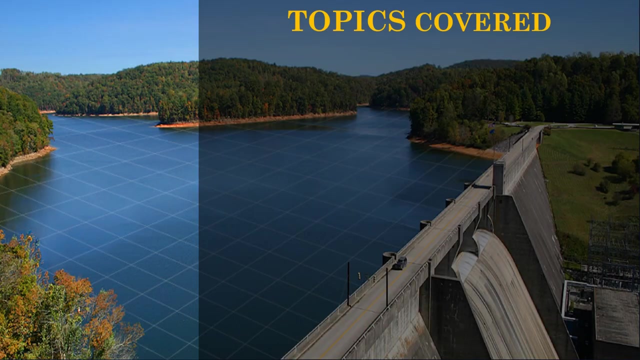 Diploma, Student, Masters and Research Fellows in Water Resource Engineering Working Professionals. Most of the course content is as per the syllabus followed by the State Universities, Government Colleges and Private Engineering Colleges and includes practical industrial inputs. Topics covered: Section 1: Introduction to Water Resources. 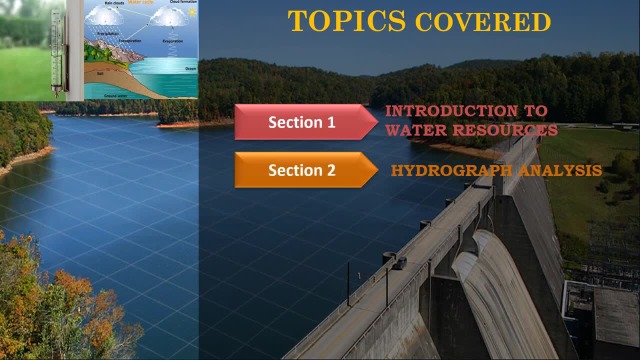 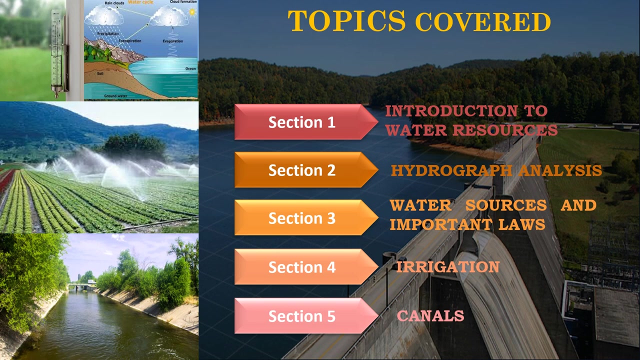 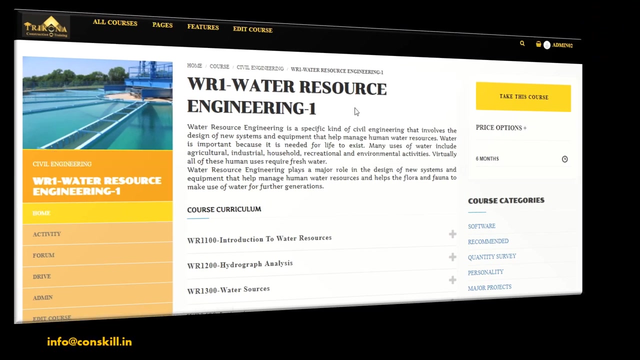 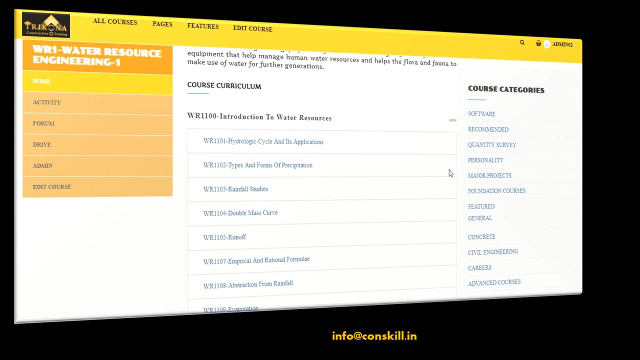 Section 2: Hydrograph Analysis. Section 3- Water Sources and Important Logistics Laws. Section 4- Irrigation. Section 5- Canals. Let's have a brief overview of Tricana Online Course Layout. Tricana Online Advantage offers you flexibility to earn credit points for timely completion of the units, excellent performance on the course, assignments and quizzes, participation in group activities or through Tricana referral system. 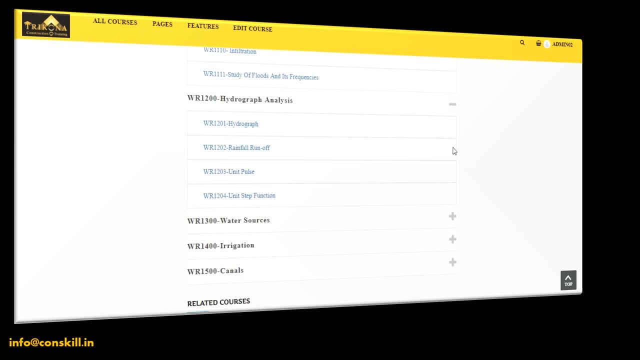 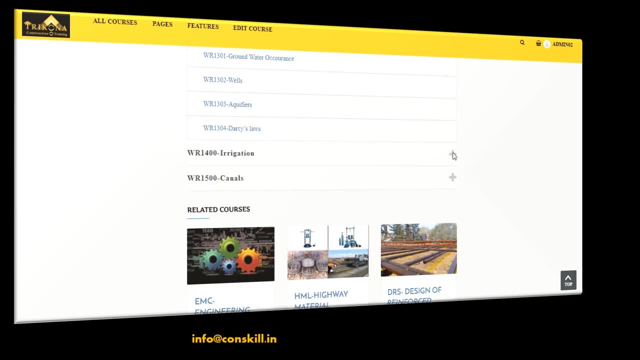 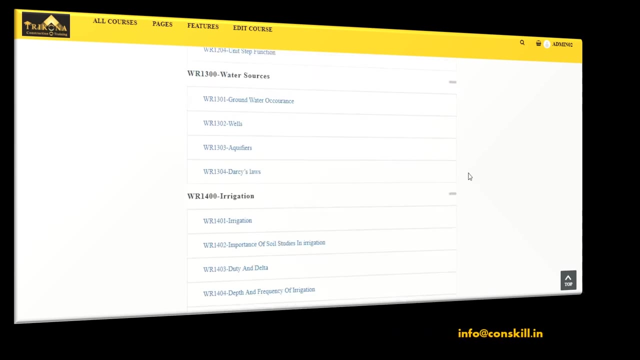 You can redeem these credits to enroll for new courses, get cash discounts on existing course or purchase additional courses. Tricana credits can give you access to higher subscription levels. You can also gift or transfer these credits to others. You can either subscribe or purchase this course.